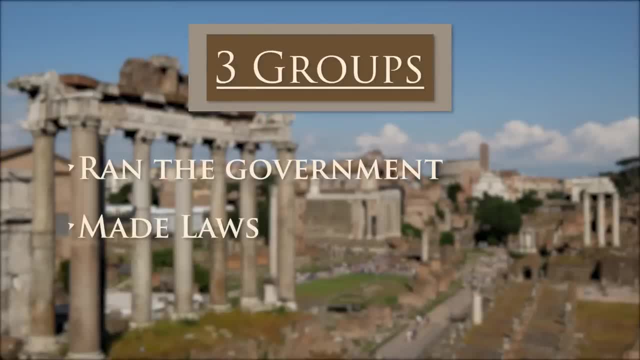 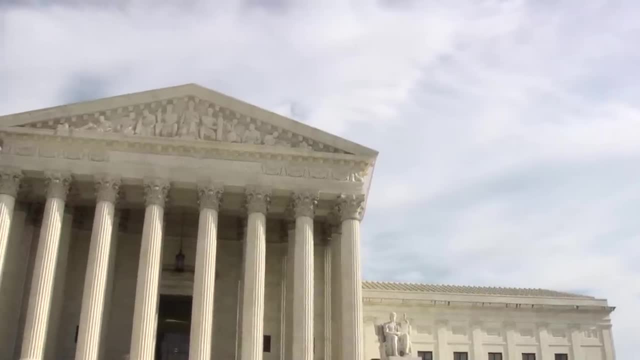 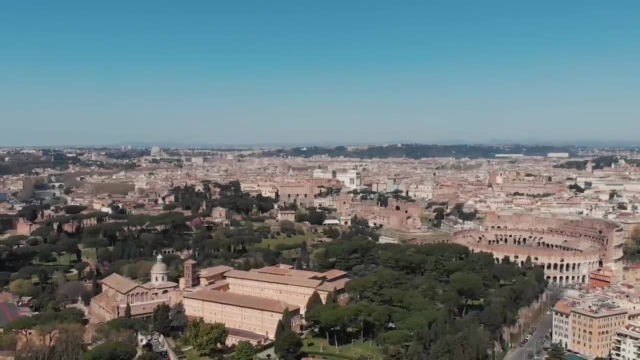 Rome's government was made up of three groups. One of the groups ran the government, Another group made the laws And a third group acted as judges. The United States government is also made up of three groups. just like Rome had Other countries used Rome as an example of how to rule and run their countries. 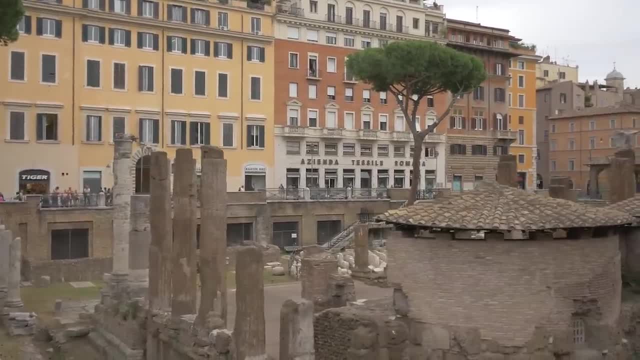 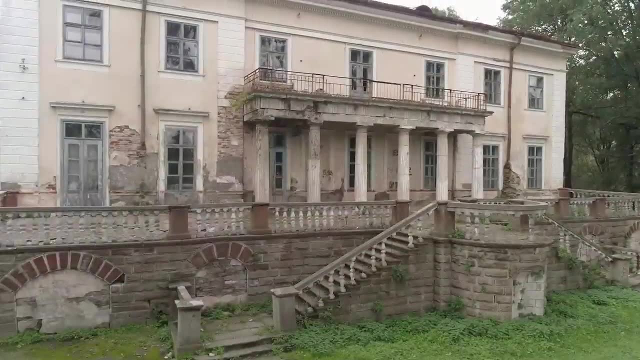 But along with Rome's success, they also had some difficulties. As Rome got bigger, the rich citizens got richer while the poor people got poorer. The rich spent their time in the city, while the poor people got poorer. They spent large sums of money on homes, gardens, slaves and luxuries. 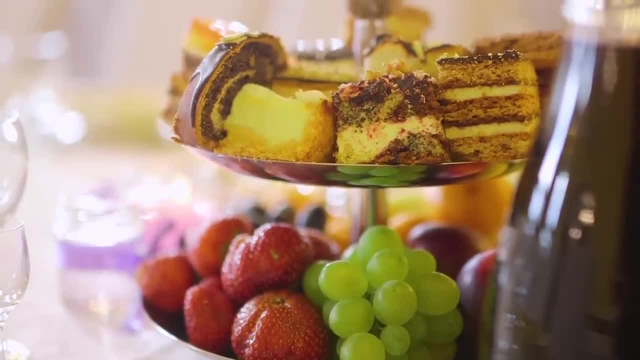 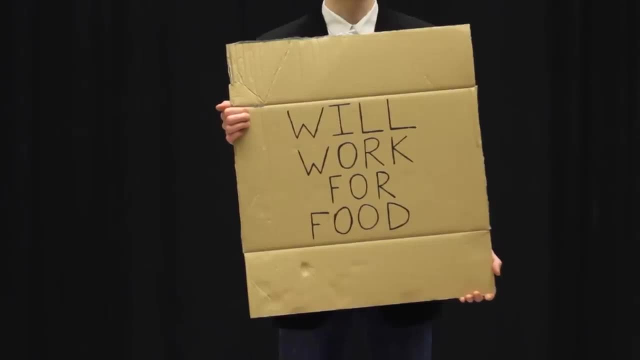 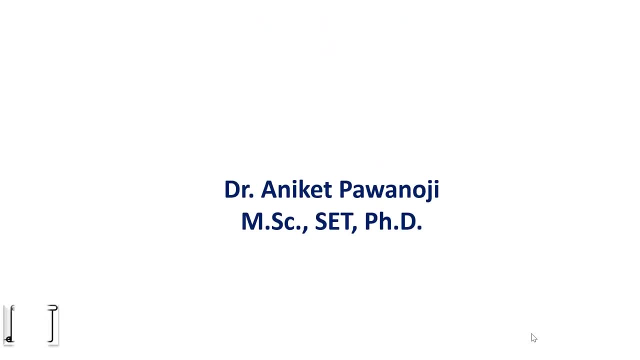 Hello friends, I am Dr Aniket Paunoji and you are watching Basic Chemistry. Welcome to the next lecture of bonding in coordination compounds. In the last lecture we have seen the postulates of molecular orbital theory and we have also seen how the bonding takes place between the central metal atom. 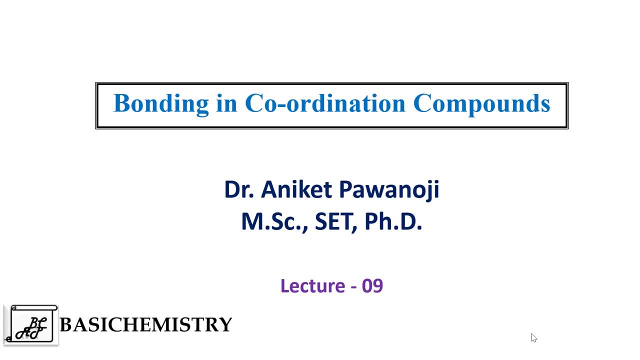 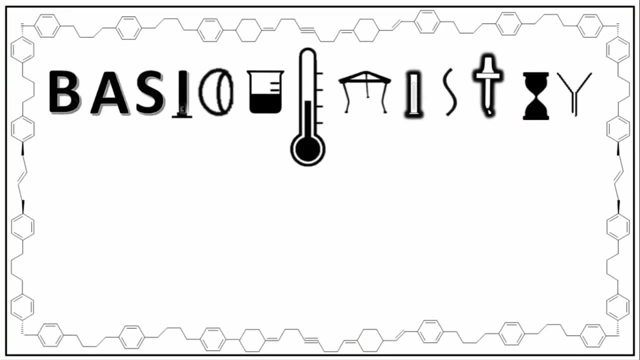 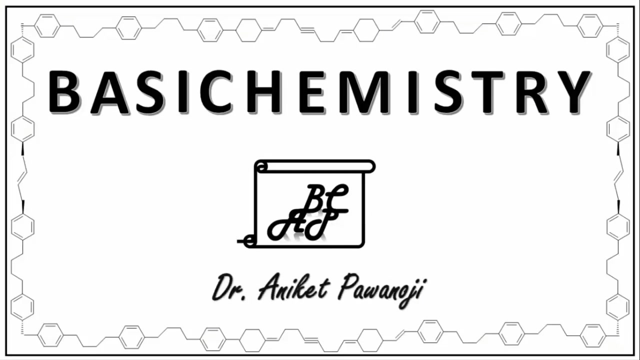 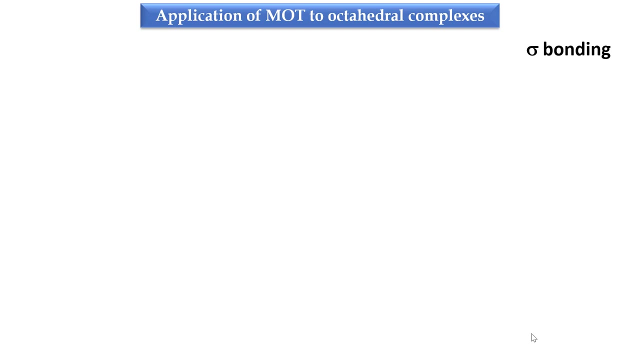 and the surrounding ligand group orbitals. In this video we will see some examples where the molecular orbital theory is applied to transition metal complexes. Let's start the video. In the last video we have seen the molecular orbital diagram for octahedral complexes consisting of sigma bonding.